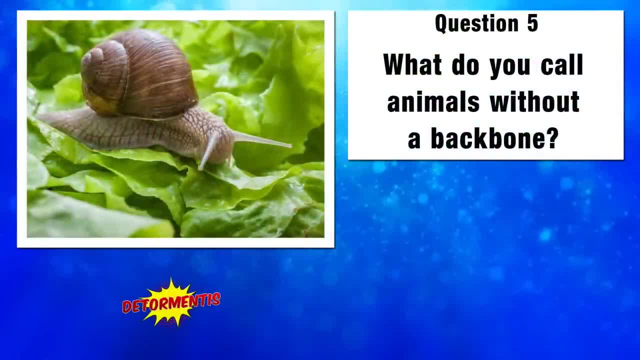 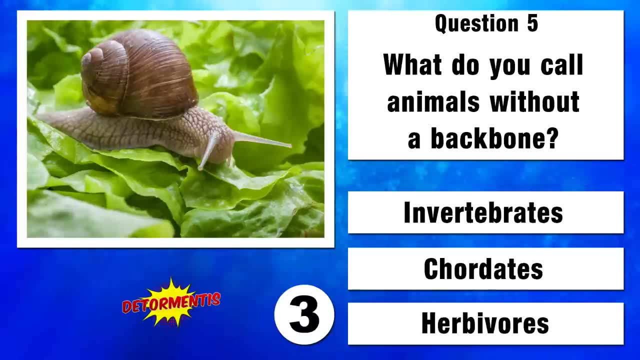 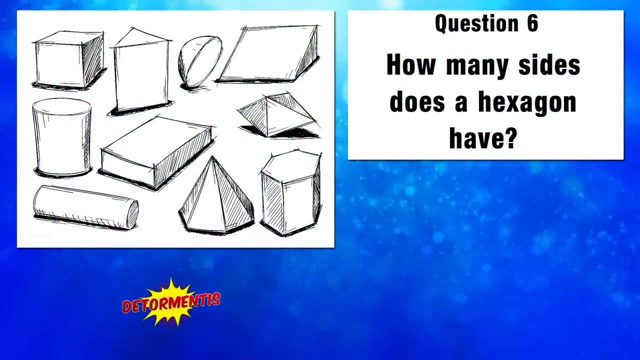 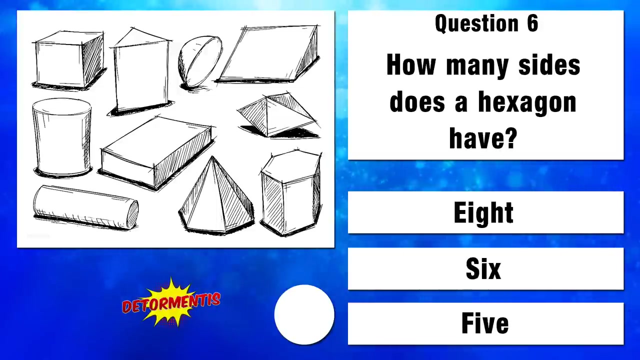 The Himalayas- Question 5.. What do you call animals without a backbone? Invertebrates, Cordates or Herbivores Invertebrates- Question 6.. How many sides does a hexagon have? 8,, 6 or 5? 6? 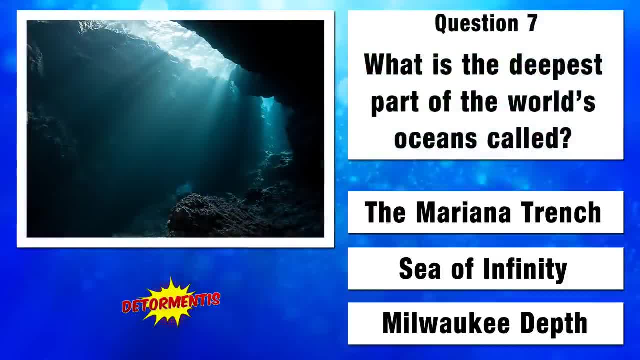 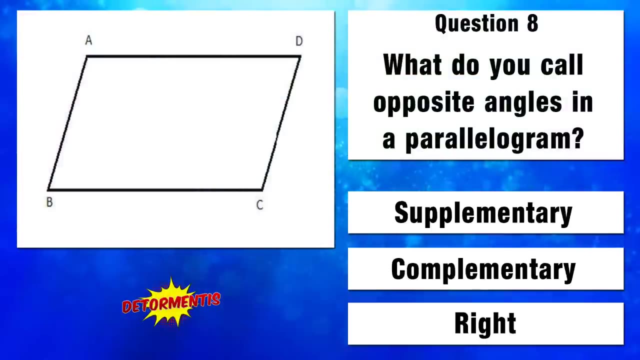 What is the deepest part of the world's oceans, called The Mariana Trench Sea of Infinity or the Milwaukee Depth, The Mariana Trench? Question 8.. What do you call opposite angles in a parallelogram- Supplementary, Complementary or Right Angles? 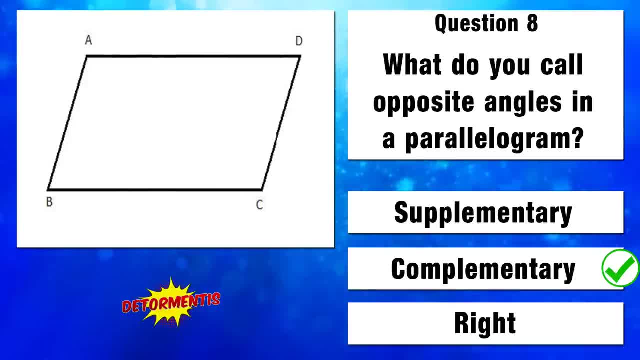 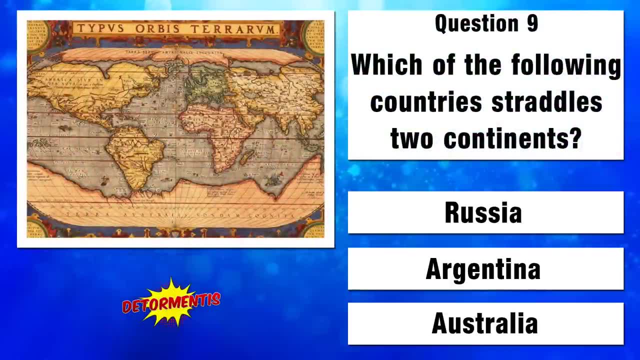 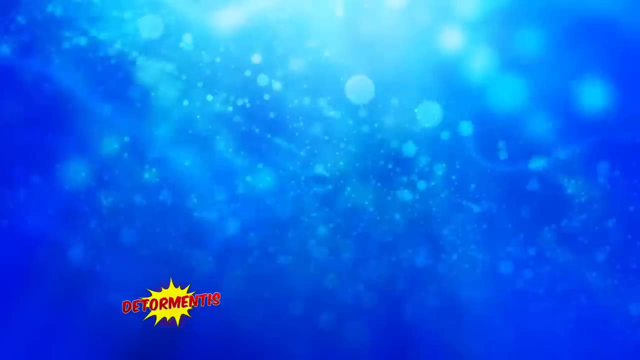 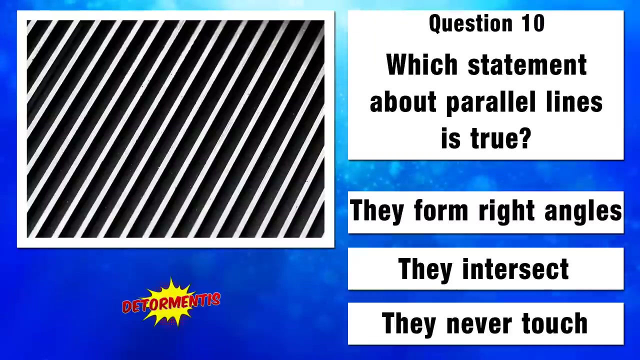 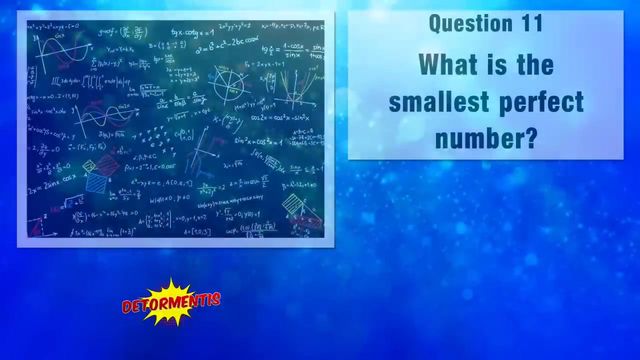 Complementary. Which of the following countries straddles two continents? Russia, Argentina or Australia, Russia- Question 10.. Which statement about parallel bounds is true? They form right angles, they intersect or they never touch. They never touch. What is the smallest perfect number? 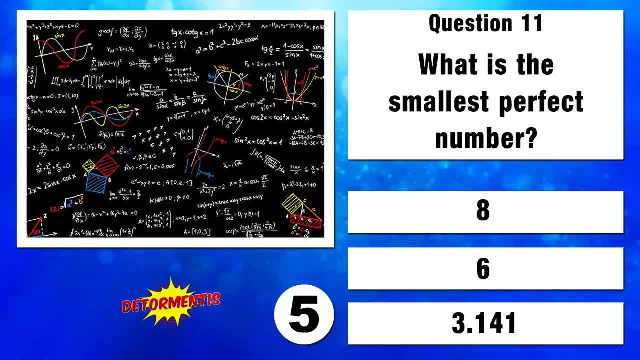 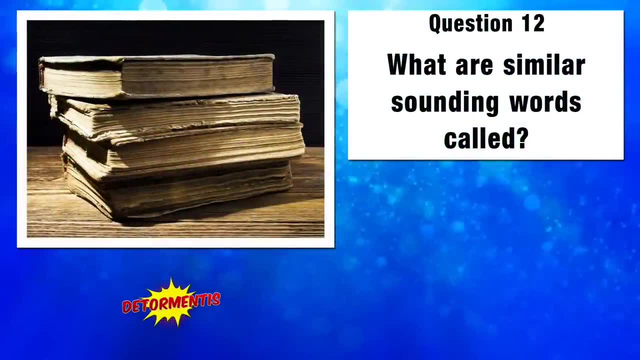 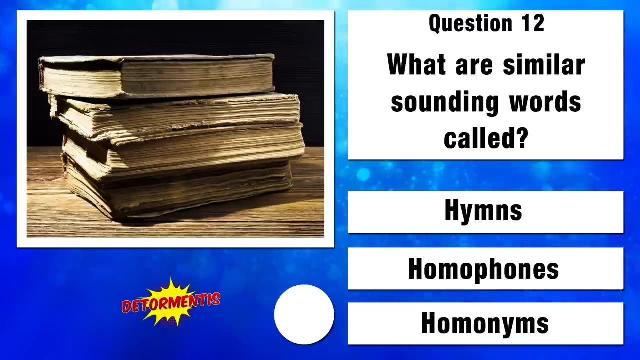 8,, 6 or 3.141? 6,, 2, 1.. What are similar sounding words called Hymns, homophones or homonyms? Hymns, homophones or homonyms, Hominems? 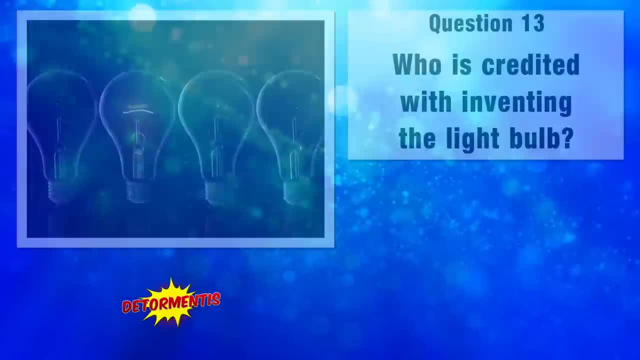 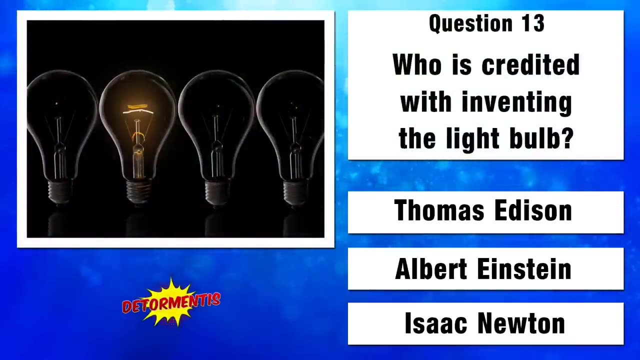 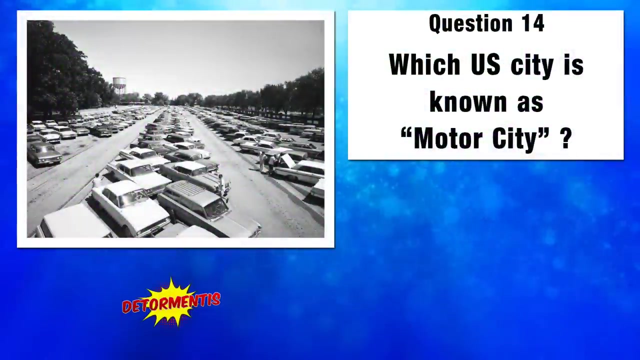 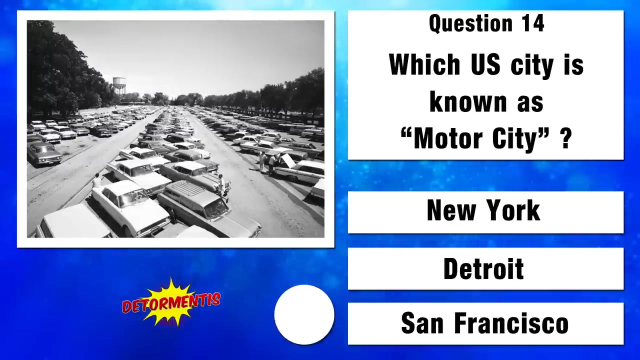 Question 13.. Who is credited with inventing the lightbulb? These are the following keywords: 1. Thomas Edison, Albert Einstein or Isaac Newton, Thomas Edison: Which US city is known as Motor City? New York, Detroit or San Francisco? 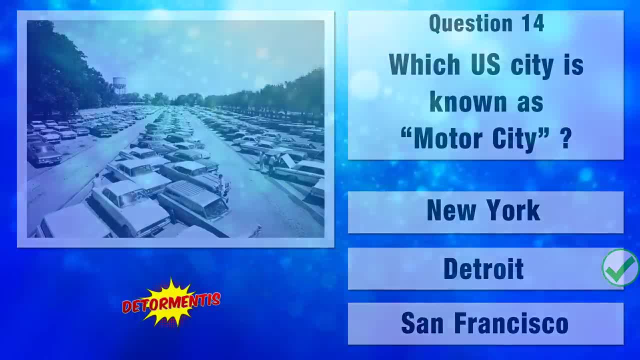 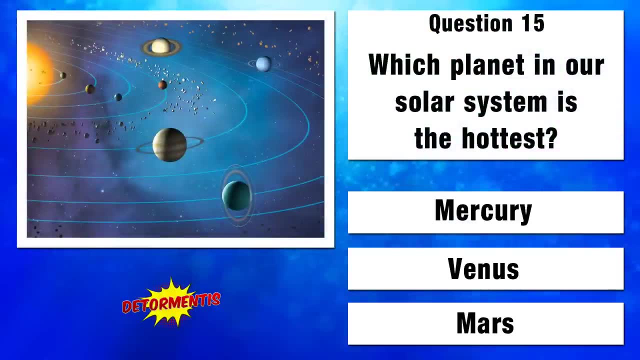 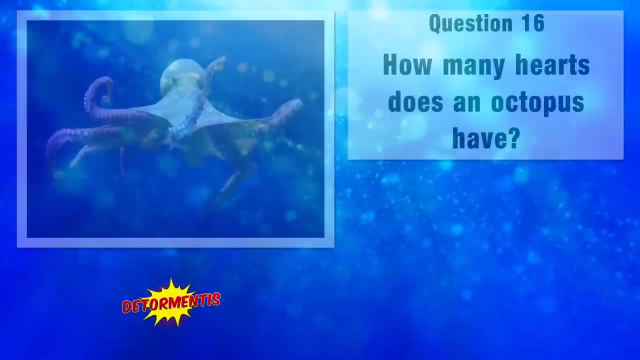 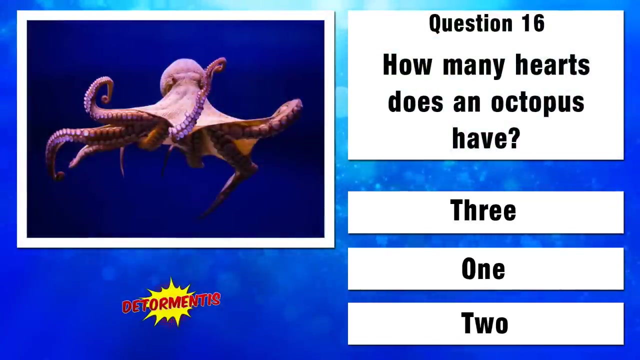 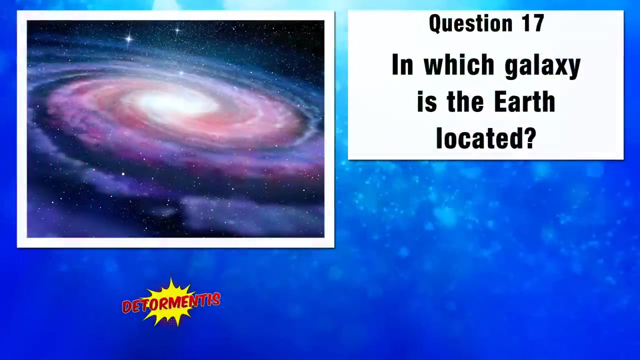 Detroit. Which planet in our solar system is the hottest? Mercury, Venus or Mars? Venus- Question 16.. How many hearts does an octopus have? 3,, 1, or 2?? 3- Question 17.. In which galaxy is the Earth located? 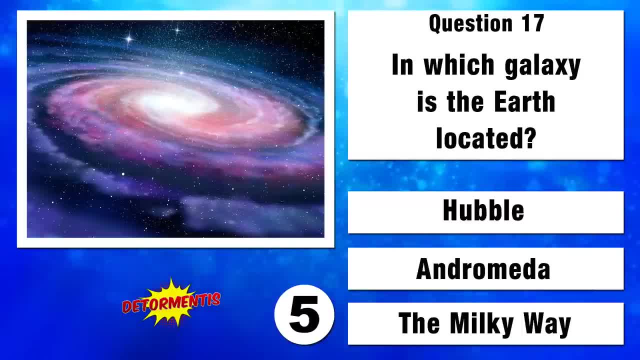 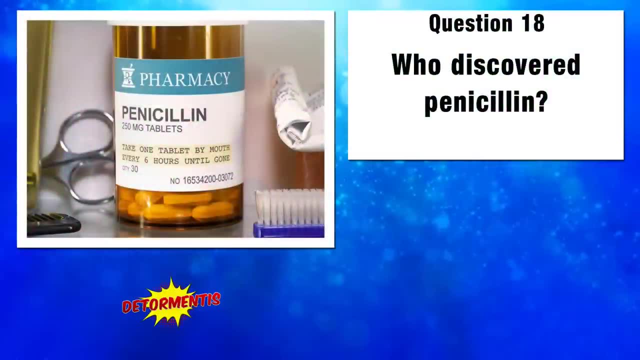 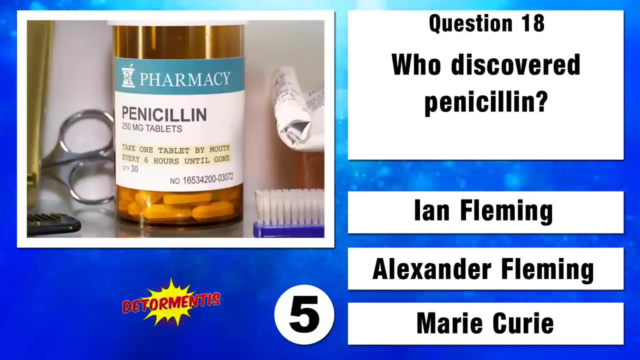 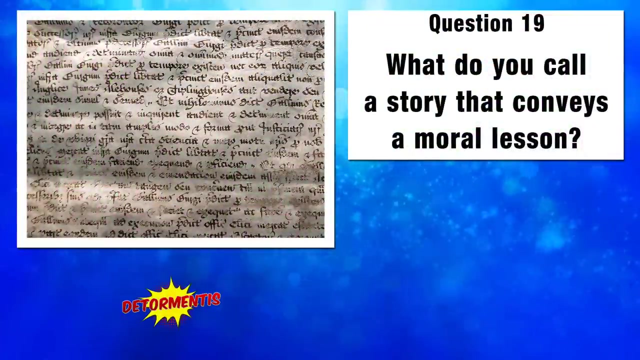 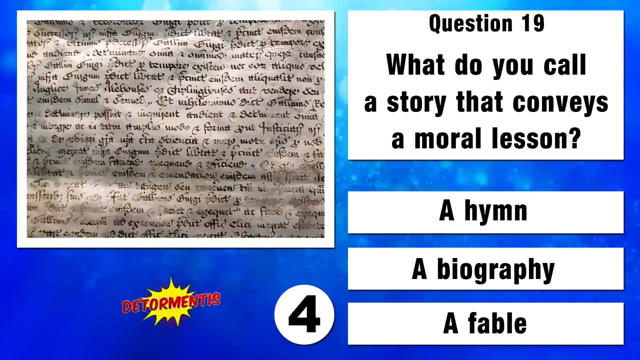 The Hubble, Andromeda or the Milky Way Galaxy? The Milky Way? Who discovered penicillin? Ian Fleming, Alexander Fleming or Marie Curie, Alexander Fleming? What do you call a story that conveys a moral lesson, A hymn, a biography or a fable? 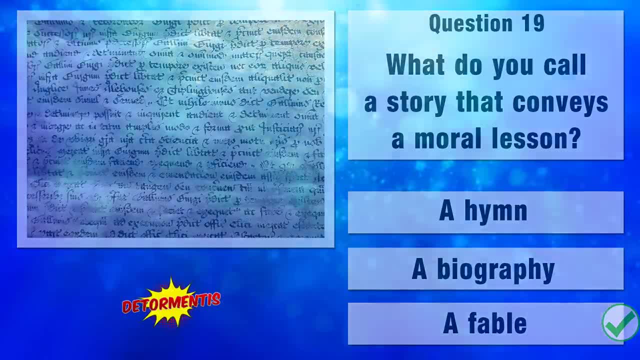 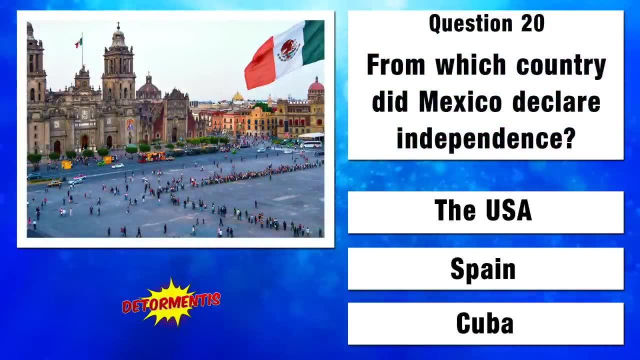 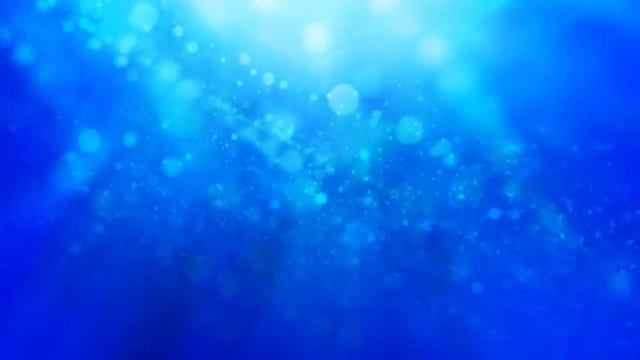 A fable. Final Question: From which country did Mexico declare independence? The USA, Spain or Cuba? Spain? Thank you so much for watching. Let me know in the comments below if you are smarter than a fifth grader and how many you've. 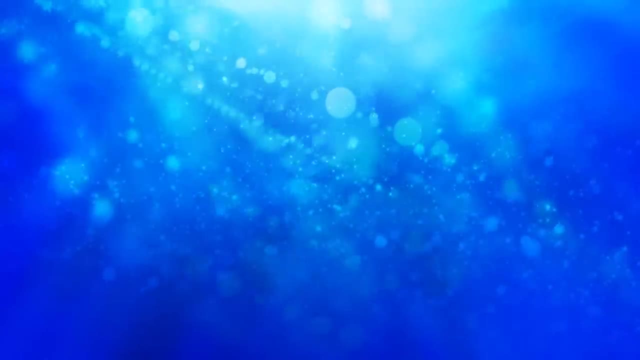 managed to answer correctly. I hope you enjoyed the video. Please leave a like. Remember to subscribe. Goodbye.